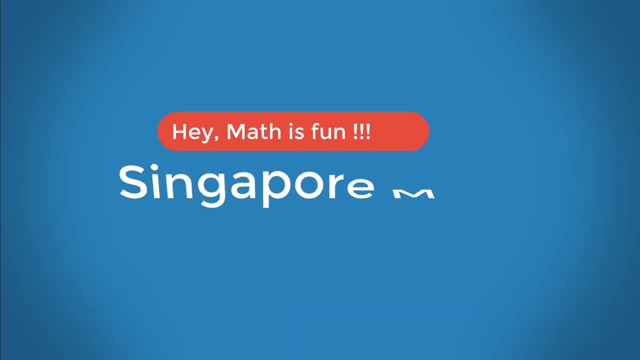 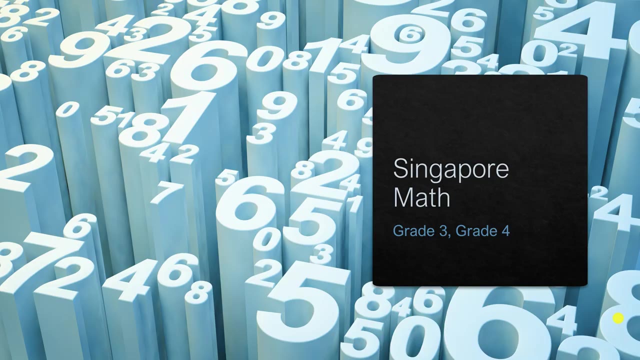 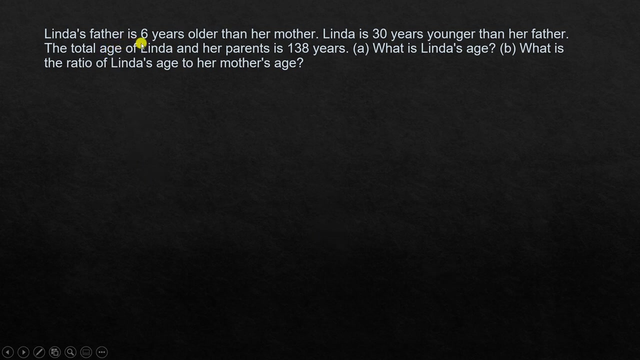 Hi everyone. we meet again with another problem to solve using Singapore math. This problem is mostly applicable for grade 3 and grade 4, but can be, you know, used by other grade students as well. The question is: Linda's father's father is 6 years older than her mother. Linda is 30 years younger than her. 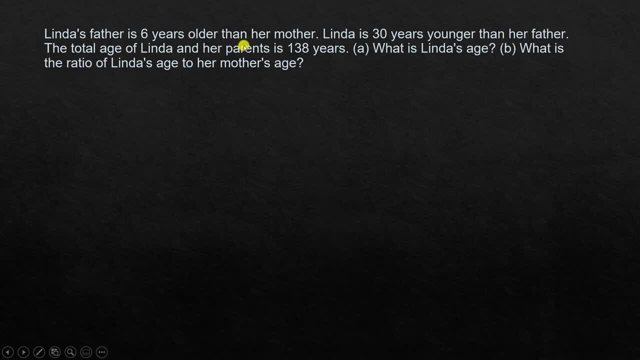 father. The total age of Linda and her parents is 138 years. What is Linda's age and what is the ratio of Linda's age to her mother's age? Let's take one statement at a time. First, Linda's father is 6 years older than her mother. 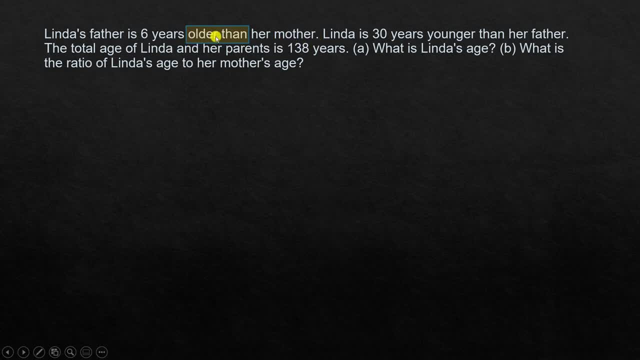 So mother comes after older than so mother. is that mother's age is the reference here. When we talk about Linda's father, mother would be the reference. Now, Linda is 30 years younger than her father. so in this case, if you look at it, when you compare Linda, the who comes after younger than it's her- 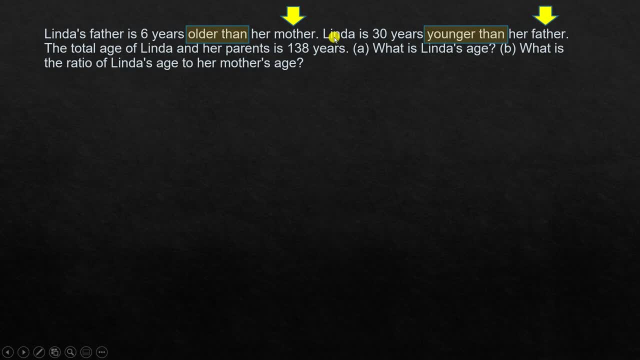 father, so he is the reference for Linda. So first let's draw a model for the first statement. Linda's father is 6 years older than her mother, So let's draw a box or model for Linda's mother. So we just draw one box and Linda's father is 6 years older than. 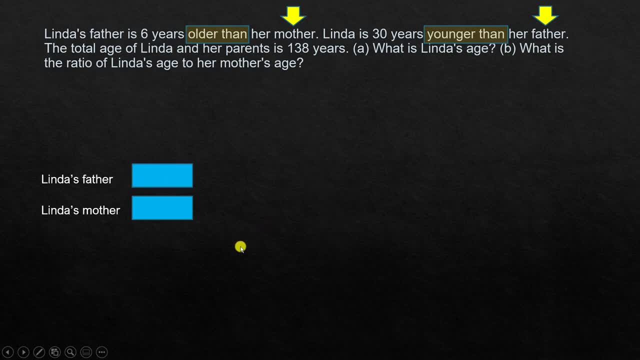 her mother. So Linda's father will be whatever Linda's mother's age plus 6.. Additionally, we have 6 here to represent that Linda's father is 6 years older than her mother. Now we come to the second statement. Linda is 30 years younger than her. 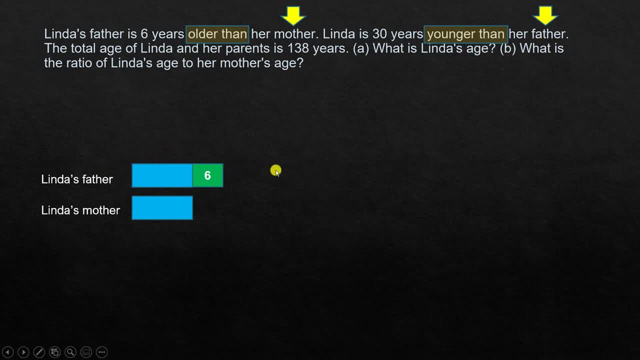 father. So this is Linda's father's age. Right, this is Linda's father's age, but we have to reduce 30 from this because she is 30 years younger than Linda's father. Now, when we try to reduce, we see that we have to reduce an arbitrary amount. but 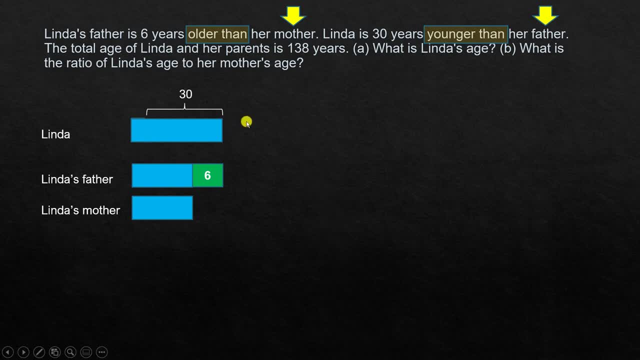 this amount has to be 30. Right, and if, when we try to do that, we can compare and see that this has to be 6, because this size here is 6, which means that the remaining size here will be 24.. So, totally, we are. 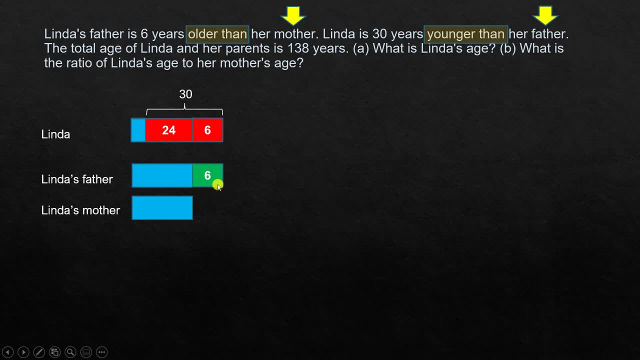 reducing 30, and we know this size is a known. this is a known quantity, so this is 6, which means the remaining size up to here is 24, and if this is 24, an equal sized box here would also be 24.. Right. 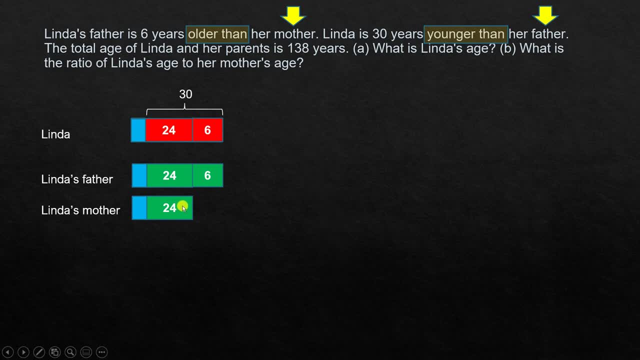 And that same applies for this as well. So, from here to here, this is going to be 24, and we know that this is not there. this has. this should be removed. Alright, so Linda's age is this much because she is 30 years younger. 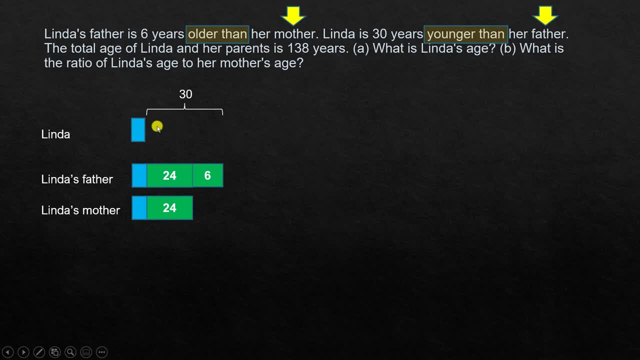 than her father. But when we try to do that, we established some known values for Linda's father and mother as well. The total age of Linda and her parents is 138 years, so this whole thing is equal to 138.. Now, when we look at it, we can clearly see that. 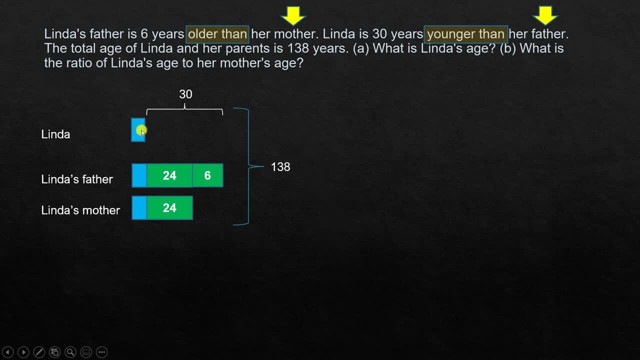 this: three are of the same size, so we have three units of the same size plus some known values. that is equal to 138.. So let's write that down: three units plus 24 plus 6 plus 24, right? three units plus 24 plus 6 plus 24 is equal to 138.. Now, when we add these three here, it becomes 54. 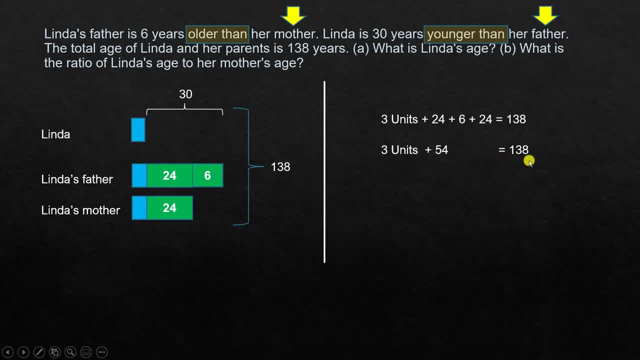 three units plus 54 is equal to 138 and we would like to remove this 54 from this side. so we minus off 54 from both sides of the equation to maintain the equality. So three units here, 54 gets cancelled away- is equal to 138 minus 54.. 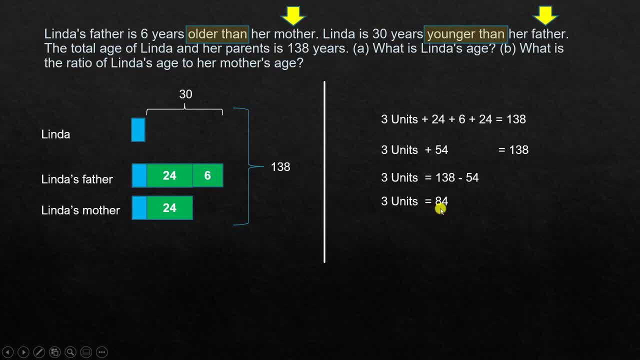 On this side. so three units is equal to 84, and one unit is equal to 84 divided by 3, which is equal to 28.. So this is Linda's age. actually, if you look at it, Linda's age is one unit, which is 28.. Now, what is Linda's mother's age? This is 28 because one unit is 28, and so Linda's mother's. 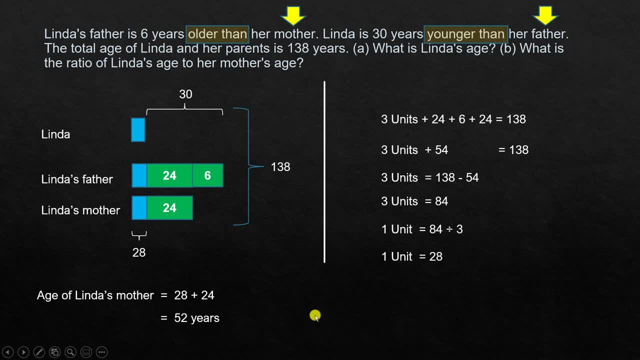 age would be 28.. Plus 24, which is 52 years old. and we know that Linda's age is 28 because it's one unit here and now we go on to the next question: What is the ratio of Linda's age to her mother's age? 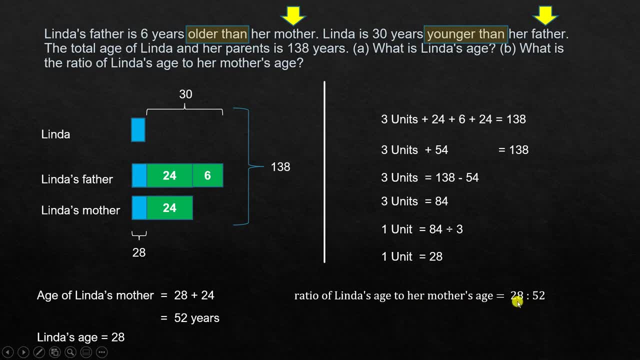 So the ratio of Linda's age to her mother's age is: Linda's age is 28, her mother's age is 52.. 28 is to 52, which you know that in ratio we will have to simplify it or divide them with the common number until we get the smallest of them. so that comes to 7 is to 13.. So that 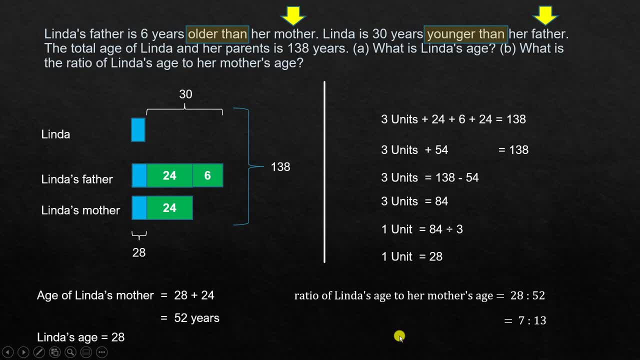 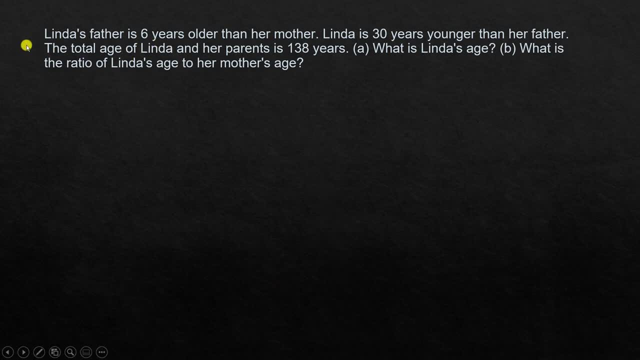 answers this question. hope this was clear. Now we move on and to try and solve this problem using algebra, The question I'll just read out once again: Linda's father is 6 years older than her mother. Linda is 30 years younger than her father. The total age of Linda and her parents is: 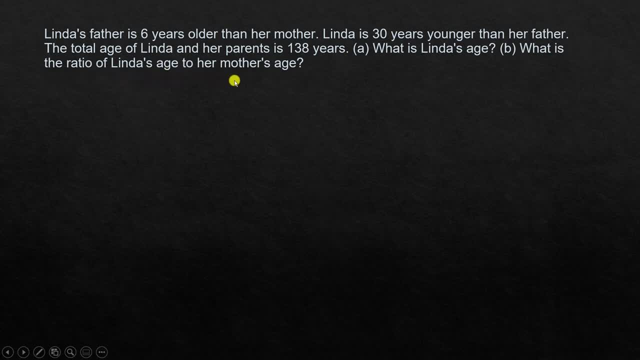 138 years. What is Linda's age? What is the ratio of Linda's age to her mother's age? So now, when we look at here, Linda's father is 6 years older than her mother. So mother comes after older than, so mother is. 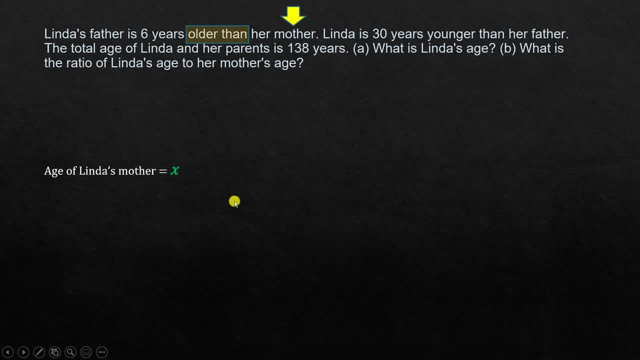 the reference. So let's assume age of Linda's mother is X. In the previous case we just drew a box, but in algebra we represent the unknown quantities. in terms of alphabets It can be anything, but generally we start using like X, Y. it could be A, B, M and anything. 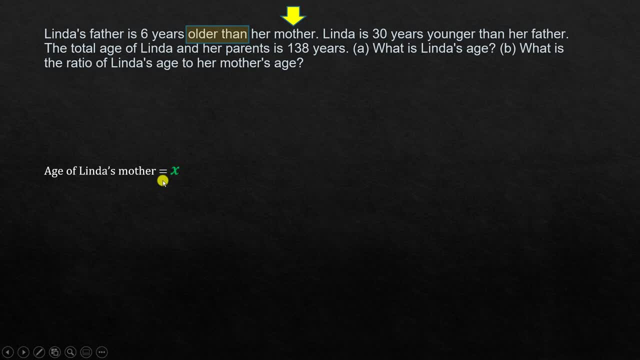 actually Right, It just means it's. we don't know the value of this. And Linda's father is 6 years older than, or more than, so he has to be. whatever is the mother's age plus 6, and Linda is 30 years younger than her brother, So father's age minus 30 will give Linda's 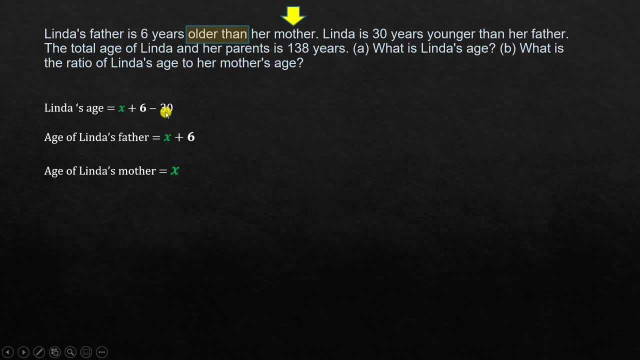 age minus 30.. So this is how we represent the age of all of these three people. Now the next statement says the total age of Linda and her parents is 138 years. So if we add these three it should come to 138.. We have to add all these three quantities so that we can bring up to 138. 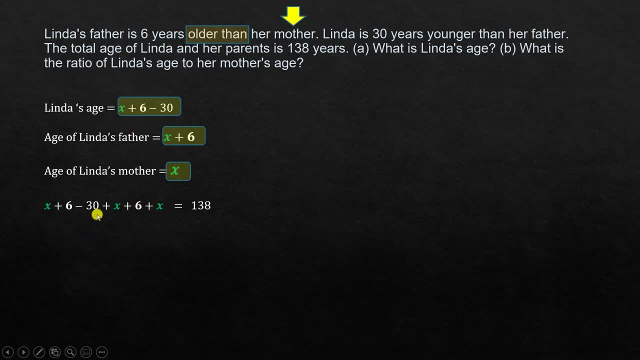 So let's write them down: x plus 6 minus 30 plus x, plus 6, which is father's age, plus x, which is mother's age, is equal to 138.. Now in this, this is an equation, So we are going to add up all the x together. there are three x's here: x plus x plus x, so 3x and 6 plus 6 is 12.. 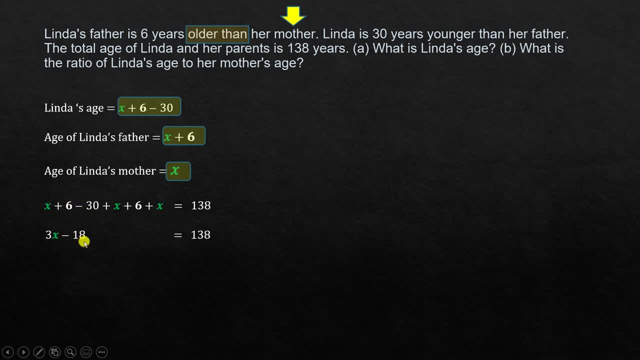 12 minus 30 would be minus 18 and that is equal to 138.. Now we have to cancel this 18 from this side. This is minus 18, so we add 18 on both sides so that this gets cancelled off. That is 3x plus x minus 12 minus 3x plus 3x equals 138. 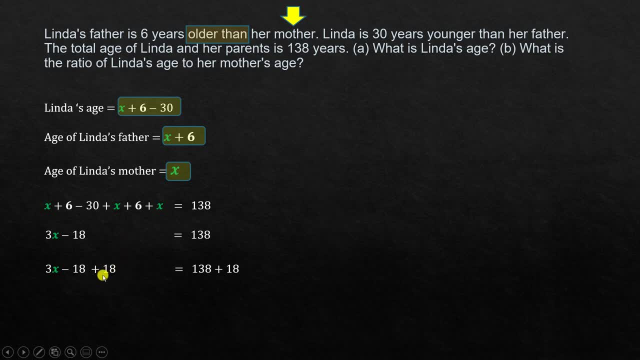 minus 18, plus 18, because we are adding plus 18. we are adding 18 here. we have to add 18 on the right hand side as well, so that the equality is not affected, right? so minus 18 and 18 gets cancelled away. so 3x is equal to 156 and x is equal to 156 divided by 3, which is 52, and we know. 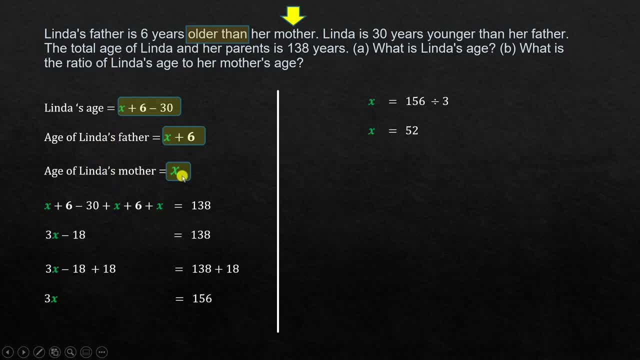 that x is age of linda's mother, so linda's mother is 52 years old and linda's mother is age of linda's mother is x, so she's 52 years old and linda's age is x plus 6 minus 30. so let's replace.